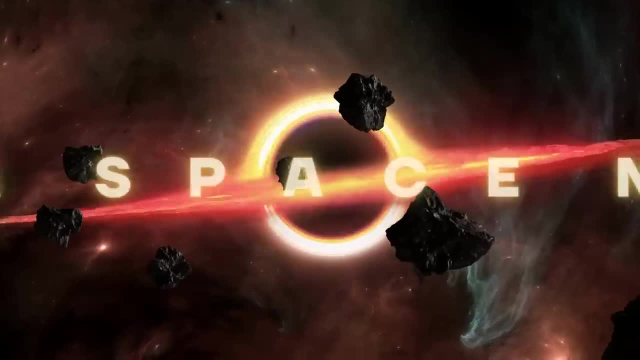 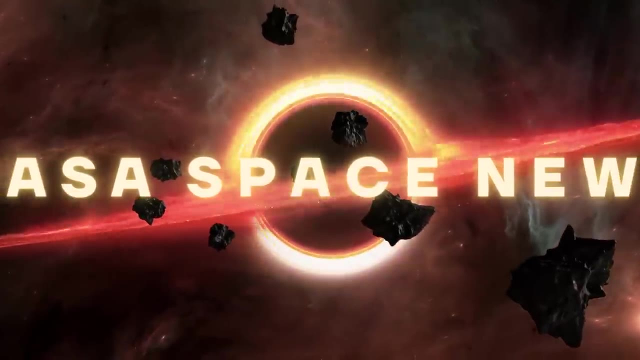 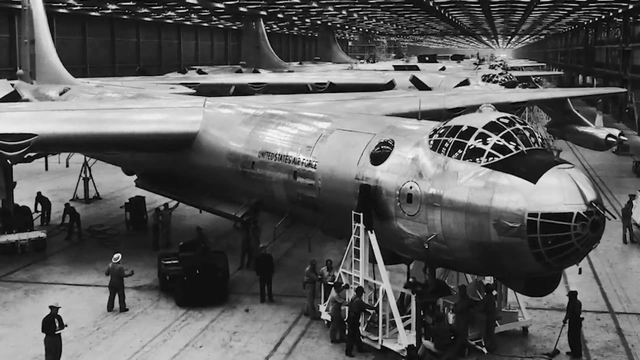 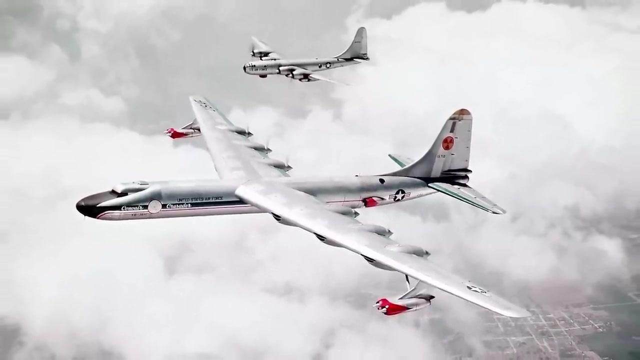 possibilities of the future of space travel. The story of nuclear propulsion begins in the 1950s, when NASA was and the United States Air Force began developing a nuclear-powered aircraft engine. The project was ambitious but ultimately cancelled due to technical difficulties and 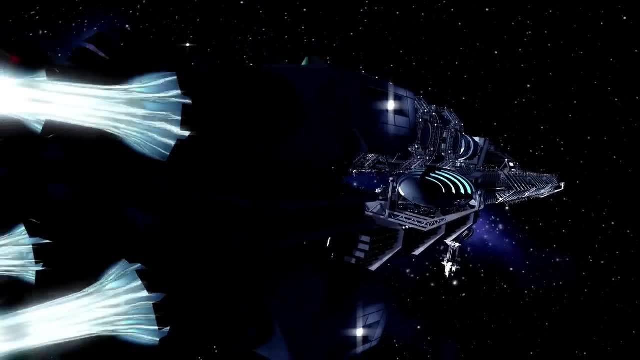 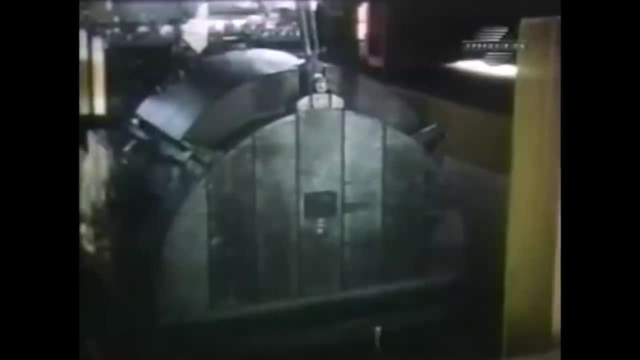 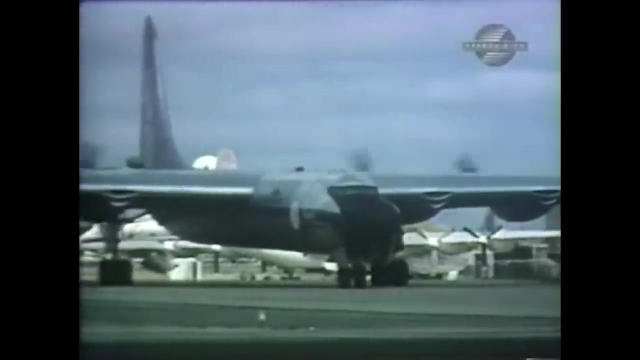 concerns about safety. However, the idea of using nuclear power for space travel never truly died. In the following decades, NASA and other space agencies continued to study the potential of nuclear propulsion for space travel. In the 1980s, NASA even conducted a test flight of a nuclear-powered aircraft, the NB-36H. 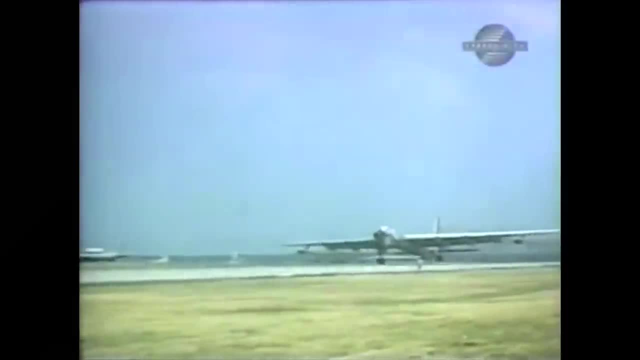 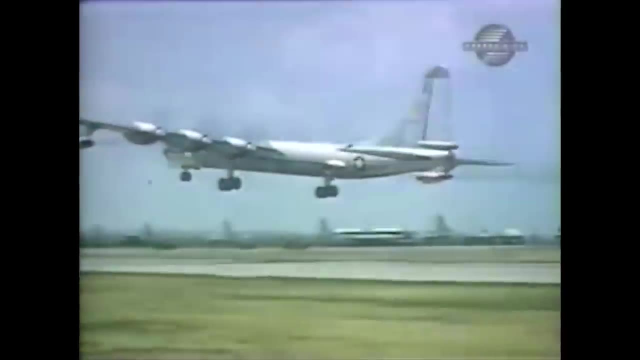 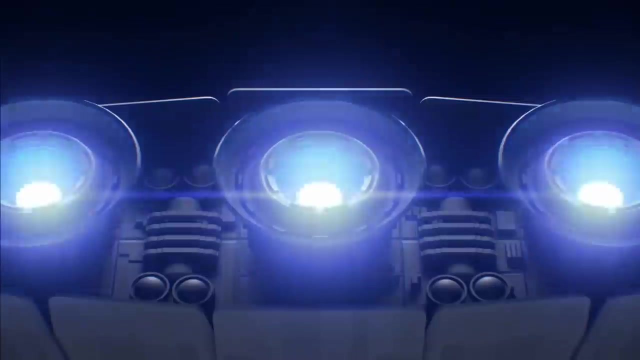 Although the flight was considered a success, the program was eventually cancelled due to budget constraints, But the seed of the idea had been planted and the potential of nuclear propulsion continued to be studied. Fast forward to today and the technology has advanced significantly. 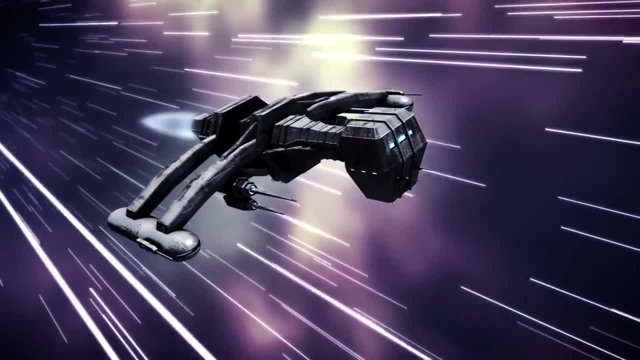 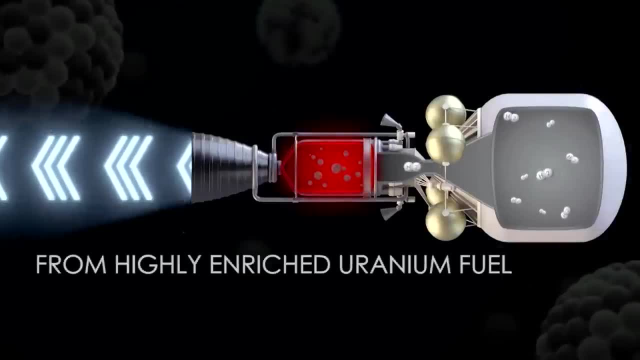 NASA's new nuclear propulsion concept is a new technology. It is based on Nuclear Thermal Propulsion, NTP, which uses a nuclear reactor to heat a propellant to create thrust. This type of propulsion could potentially cut the travel time to Mars from months to. 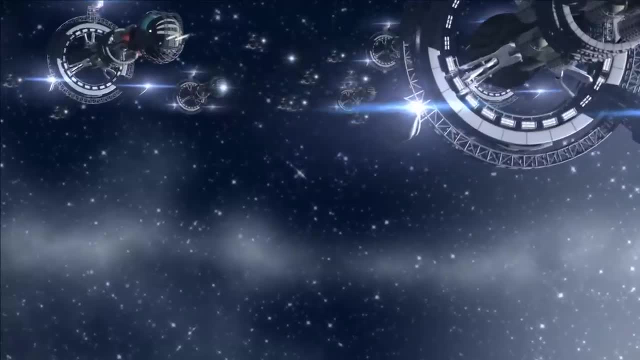 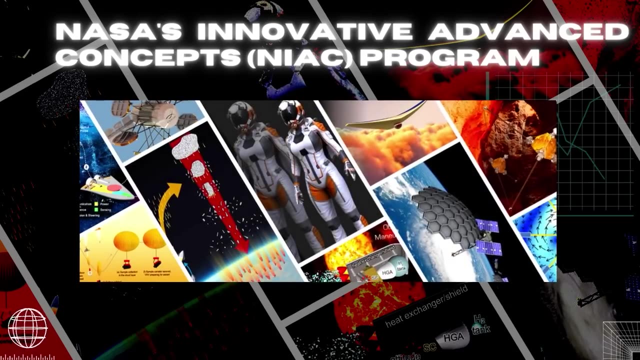 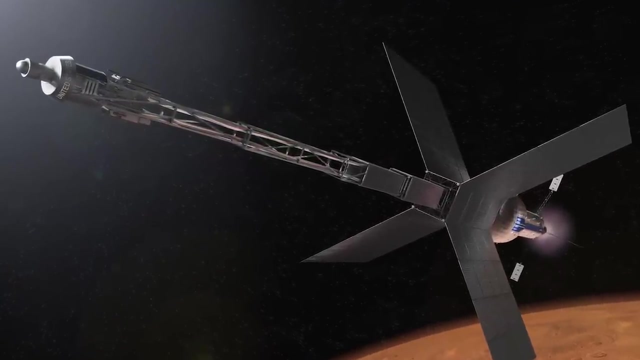 just 45 days. This is a significant advancement in space travel and could greatly benefit future missions to Mars and other planets. NASA has recently selected a new nuclear propulsion concept for phase-eye development. It is part of its Innovative Advanced Concepts program for 2023.. 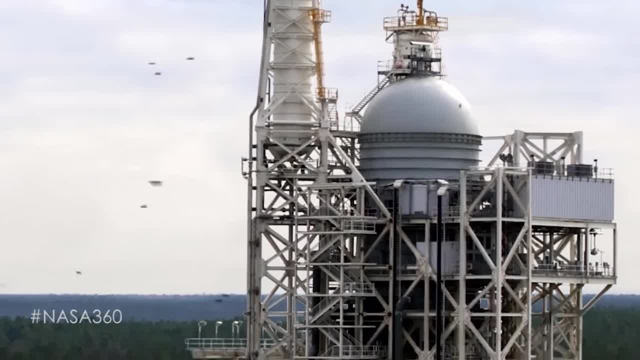 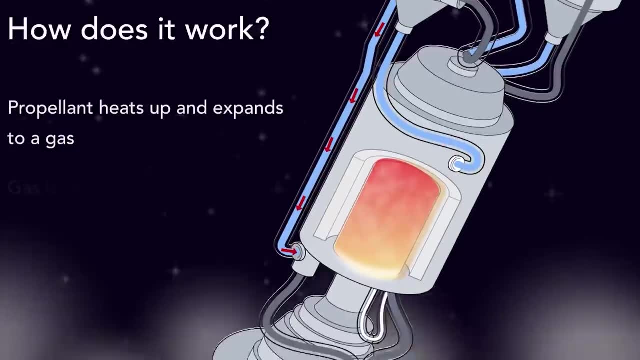 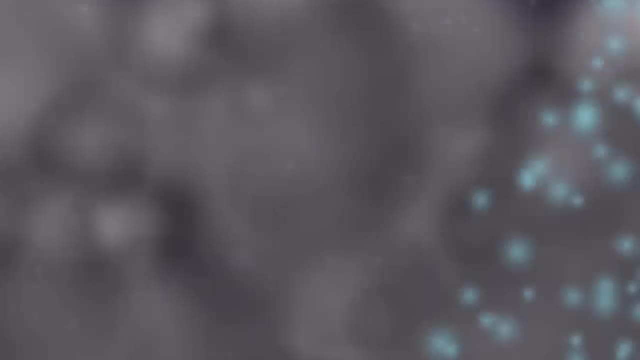 The concept called the Nuclear Thermal and Nuclear Electric Propulsion- NTP or NEP concept is a new class of bimodal nuclear propulsion system that uses a wave rotor topping cycle. The scientist behind the proposal, Professor Ryan Goss from the University of Florida. 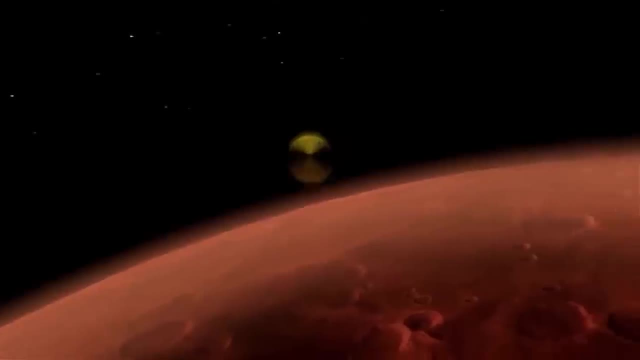 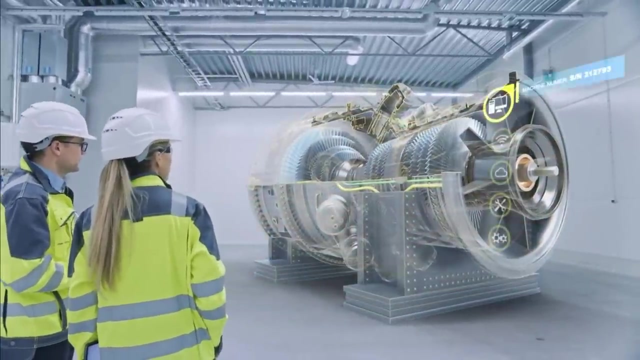 believes that it could reduce travel time to Mars to a mere 45 days. The project is currently under development. The project is currently under development. The project is currently under development. The new proposal titled Bimodal NTP-NEP, with a Wave Rotor Topping Cycle, is one of. 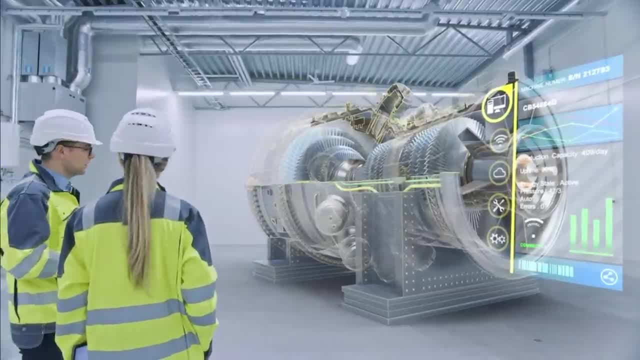 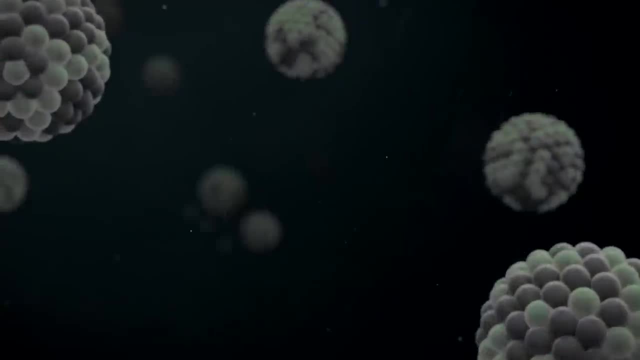 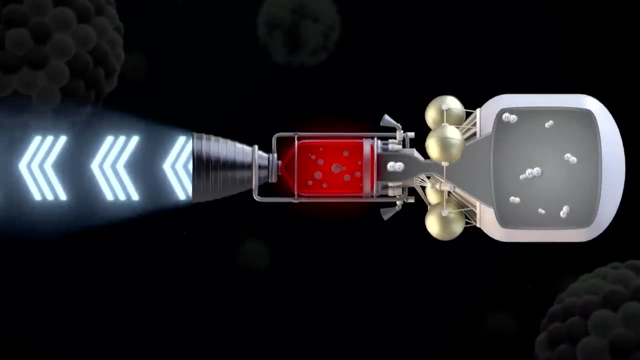 14, selected by the NAC for phase-eye development. It received a grant of the tune of $12,500 to research and develop the technology required. This concept combines the advantages of Nuclear Thermal Propulsion- NTP- and Nuclear Electric Propulsion- NEP- by using a solid-core NAVA reactor. 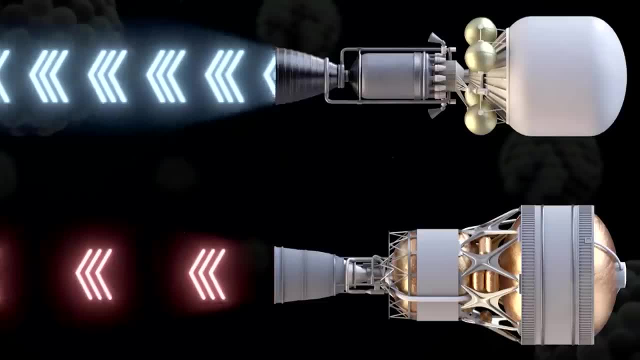 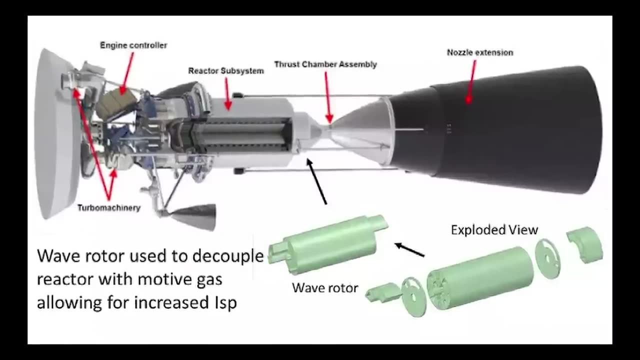 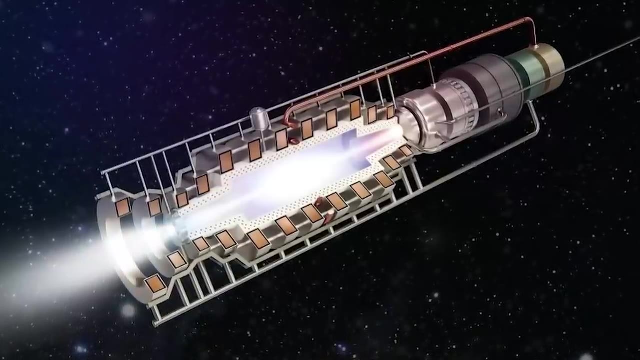 It provides a specific impulse of 900 seconds, twice the performance of existing chemical rockets. Additionally, the concept proposes using a wave rotor to compress the reaction mass further, which could deliver thrust levels comparable to a NAVA-class NTP concept with a higher ISP of 1400 to 2000 seconds. 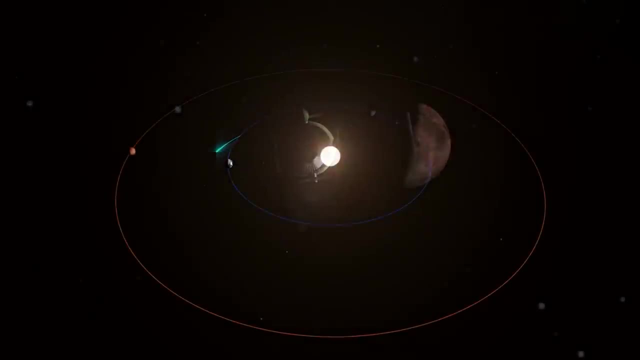 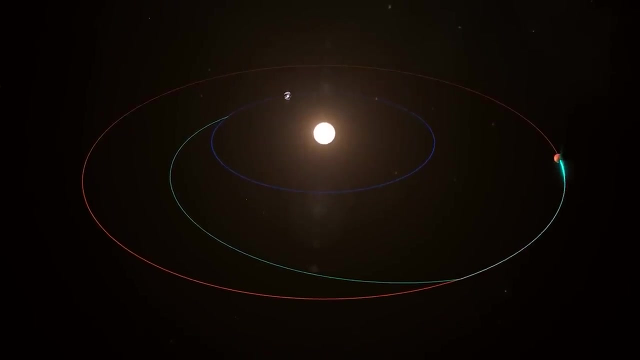 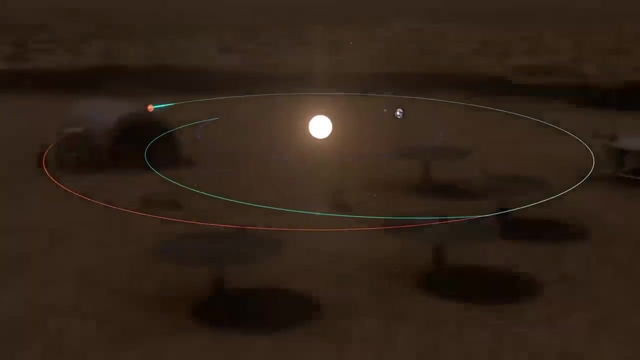 Combining this with an NEP cycle would produce even higher thrust levels, resulting in a drastic reduction in travel time to Mars. The project is currently under development. This new concept is just one of the many exciting innovations being considered by NASA's NIAC programme, which aims to identify and fund advanced concepts that could potentially 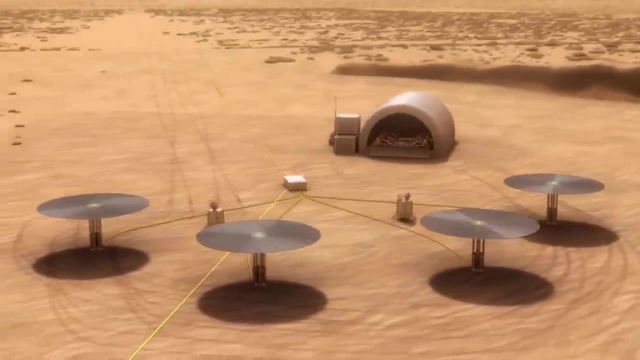 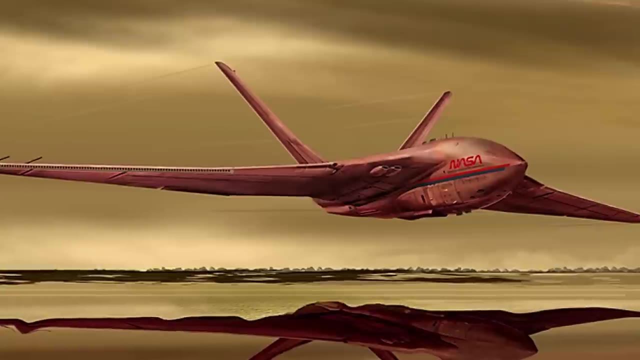 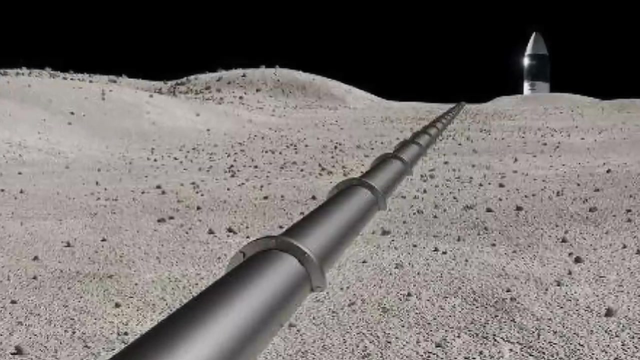 change the way we think about space exploration. Other concepts awarded a grant by the programme include a hybrid aircraft concept called Titan Air that could collect samples from the seas of Saturn's moon Titan, and a concept for a lunar pipeline that could improve the efficiency of oxygen delivery for NASA's NASA Space. 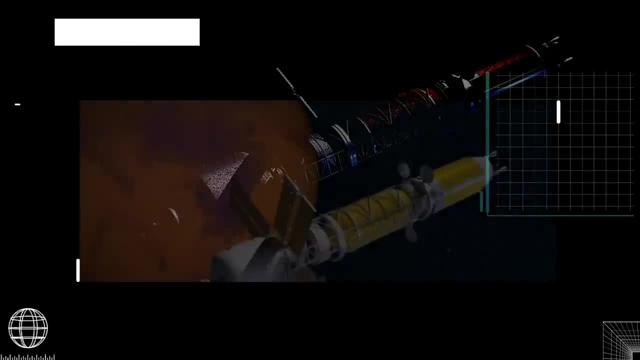 Terra mission. It is also possible to use such a new technology as the UN launch pad to affect the NFL's mission in space. The project would be a great opportunity for NASA's upcoming Artemis Moon missions. The new technology might also help present the potential implications of the new technology. 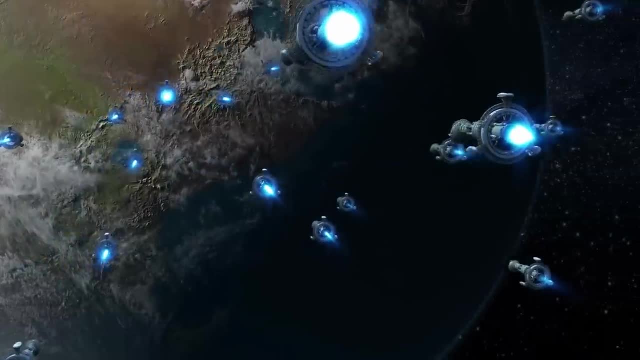 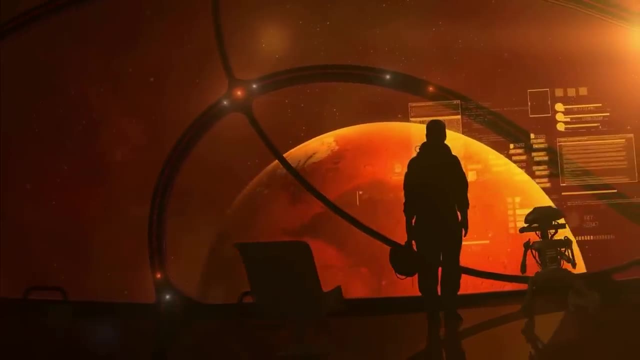 as a key part of the NASA space technology. Imagine being able to send humans to Mars in a fraction of the time it currently takes. This would greatly benefit the scientific research that could be conducted on the red planet, as well as the potential for colonising Mars in the future. 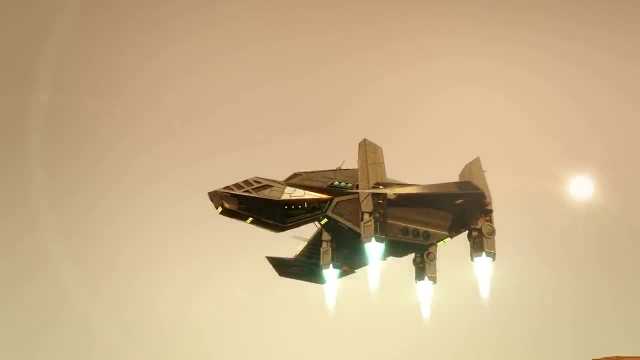 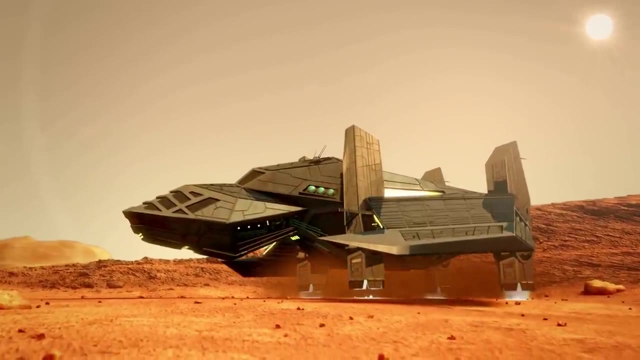 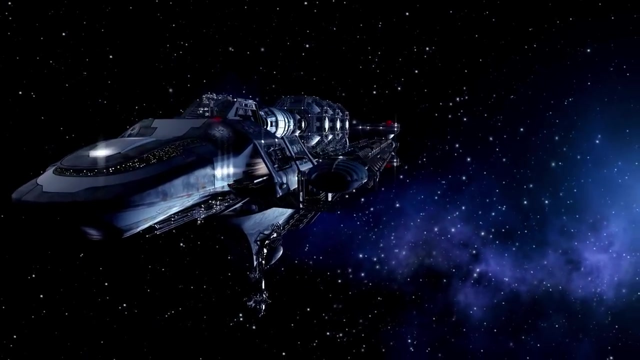 It is also possible to produce multiple Martian planets, greatly reduce the amount of resources needed for a mission, making it more cost-effective. But it's not just Mars that stands to benefit from this new technology. Nuclear propulsion could also greatly benefit missions to other planets and even other star systems. 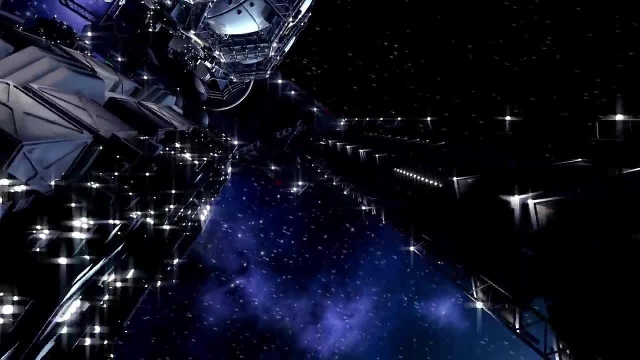 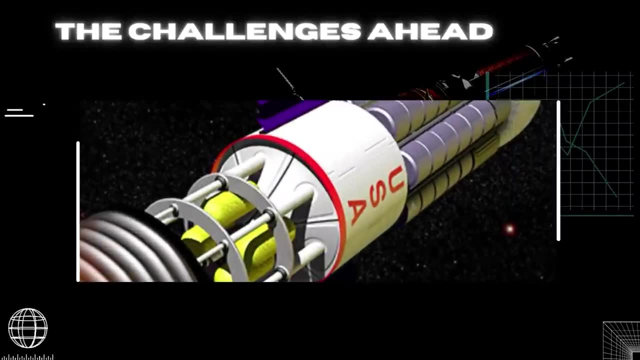 With the ability to travel faster and farther than ever before, the possibilities for exploration are truly endless. Of course, as with any new technology, there are challenges that must be overcome before nuclear propulsion can become a reality. One of the biggest challenges is safety. 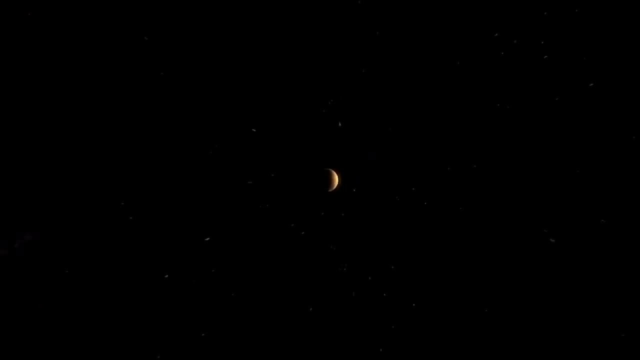 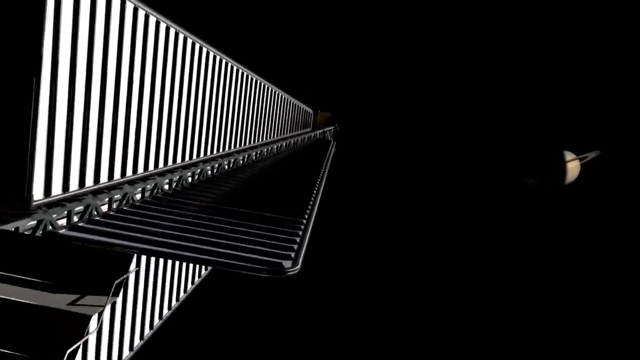 The safety of the crew and the public must be ensured, and the potential risks associated with nuclear propulsion must be thoroughly evaluated. Additionally, there are also concerns about the environmental impact of nuclear propulsion. The most important thing is to ensure that the environment is safe. 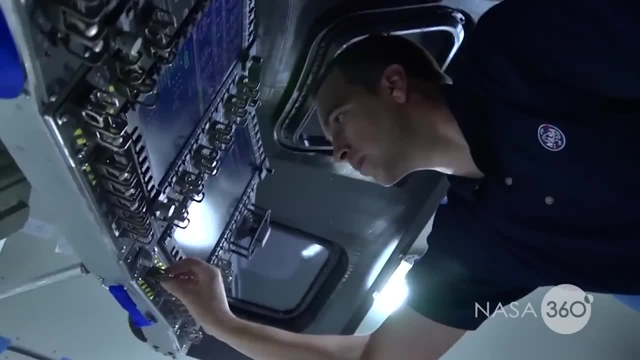 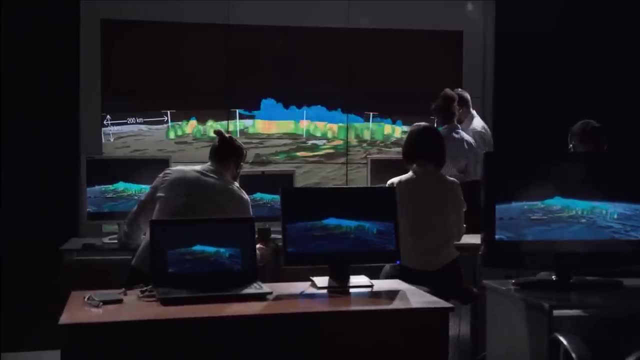 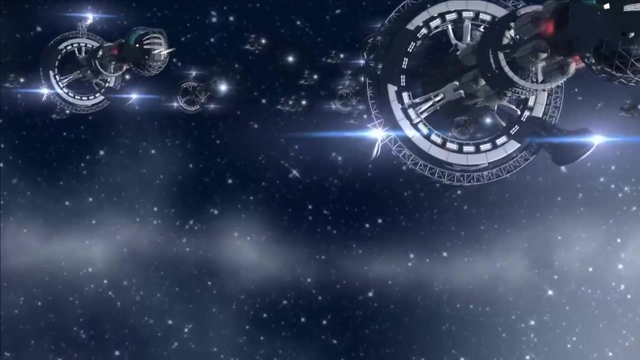 and that the environment is protected. Despite these challenges, the potential benefits of nuclear propulsion are too great to ignore. NASA and other space agencies are continuing to invest in research and development to make this new technology a reality. And as we continue to make progress in this field, 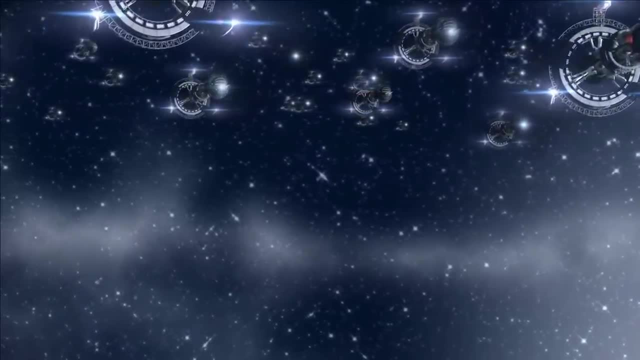 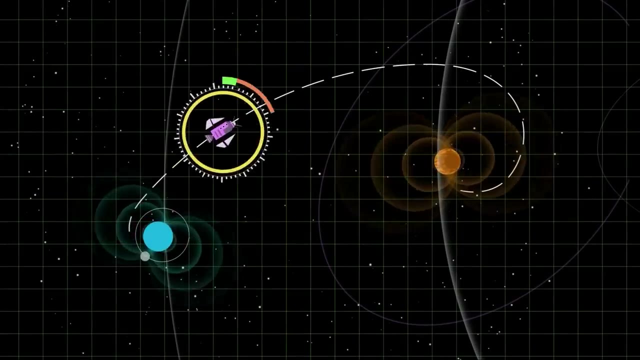 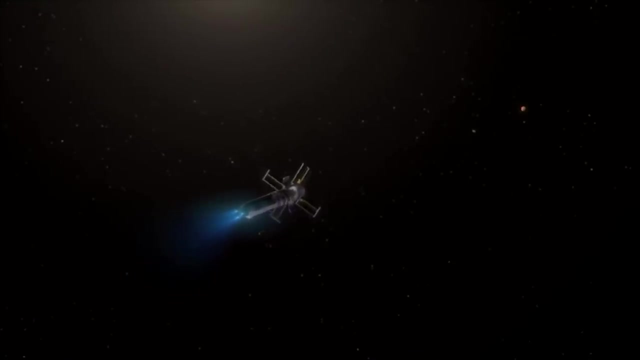 the future of space travel looks brighter than ever before. The idea of traveling to Mars in just 45 days may have once seemed like science fiction, but thanks to NASA's recent announcement of a new nuclear propulsion concept, it may soon become a reality. 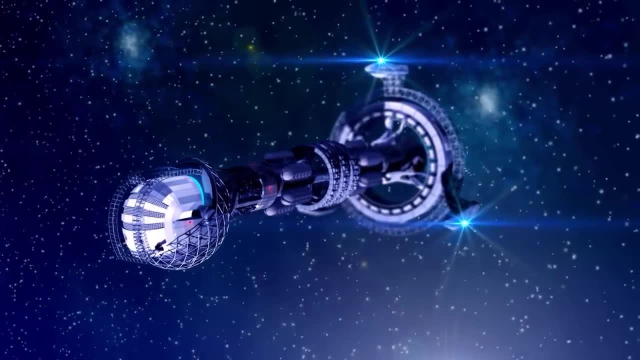 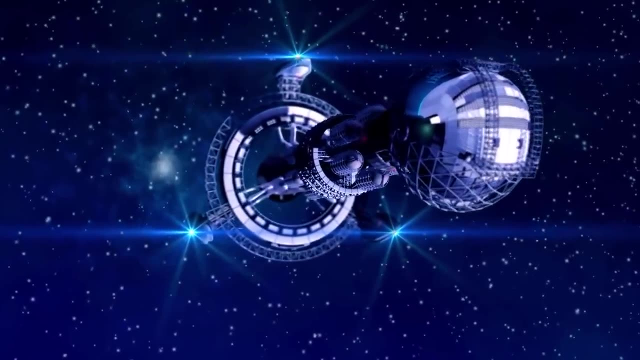 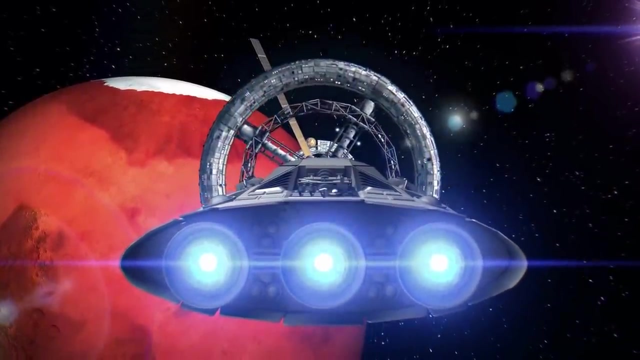 This new technology has the potential to revolutionize the way we think about interplanetary travel, and the possibilities for exploration are truly endless. While there are challenges that must be overcome, the potential benefits of nuclear propulsion are too great to ignore The future of space travel. 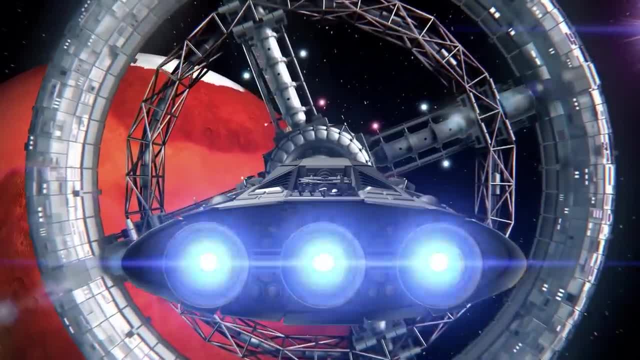 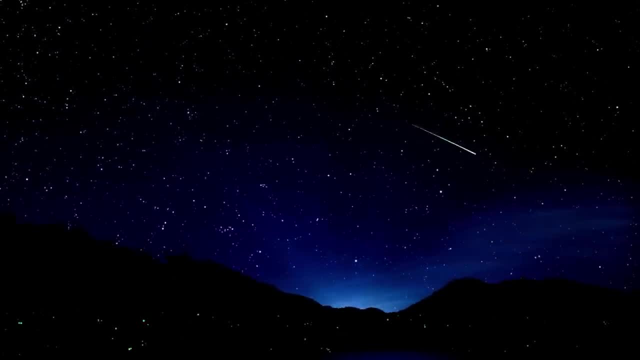 is an exciting and ever-evolving field, and we can't wait to see what the next chapter holds. So stay tuned and keep your eyes to the skies as we continue to explore the vast expanse of the Universe. Thank you for watching this video. 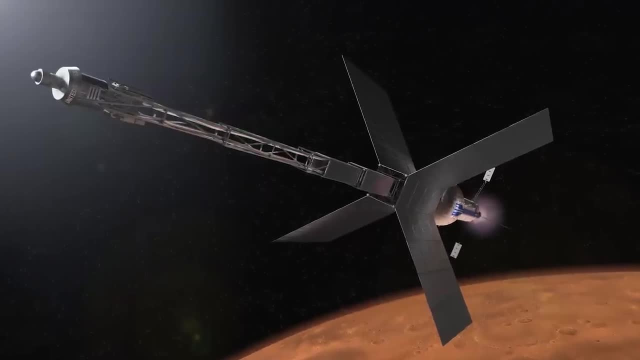 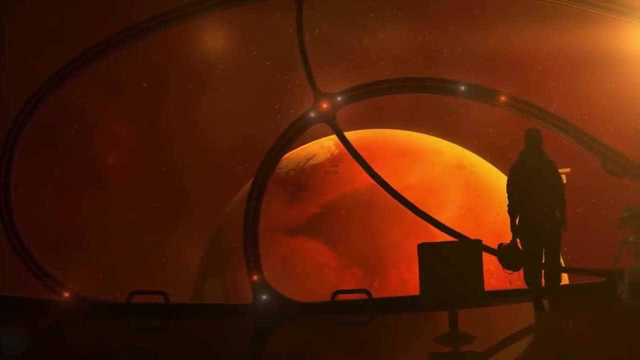 about NASA's recent announcement of a new nuclear propulsion concept. We hope that you found it informative and exciting. The future of space travel is an ever-evolving field and we are glad that you have joined us in this journey of discovery. We would like to extend our gratitude. 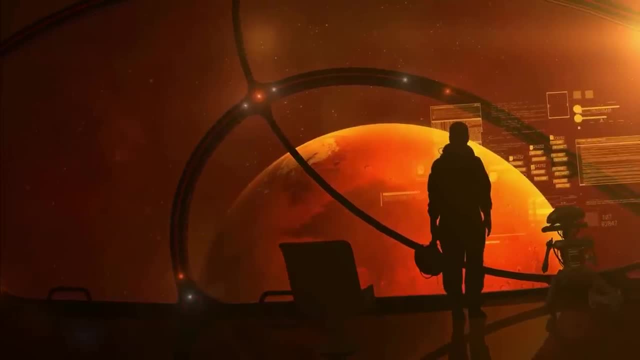 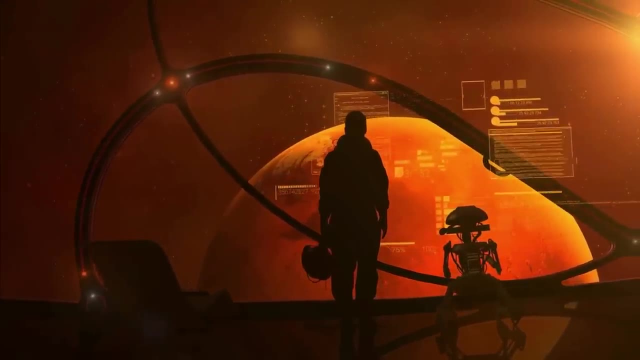 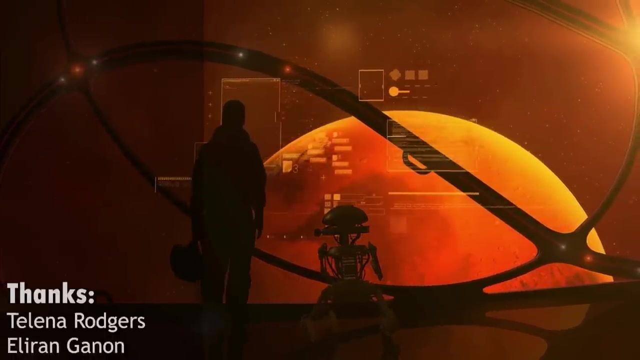 for your ongoing support and we would greatly appreciate it if you could share this video with your friends and family. Thank you. The possibilities of what we can achieve in space are endless and together we can be a part of shaping the future of space exploration. 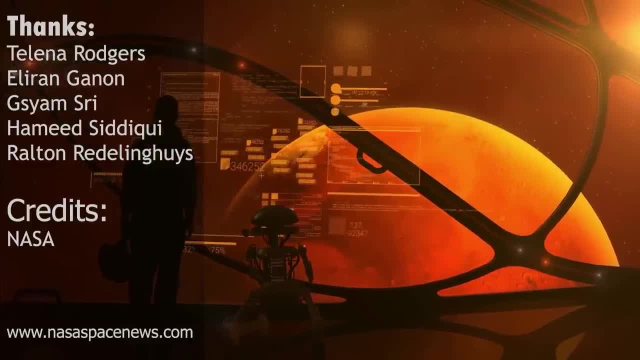 Thank you again and until next time, keep reaching for the stars.